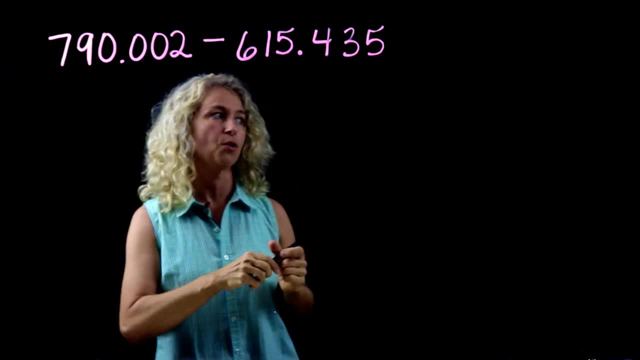 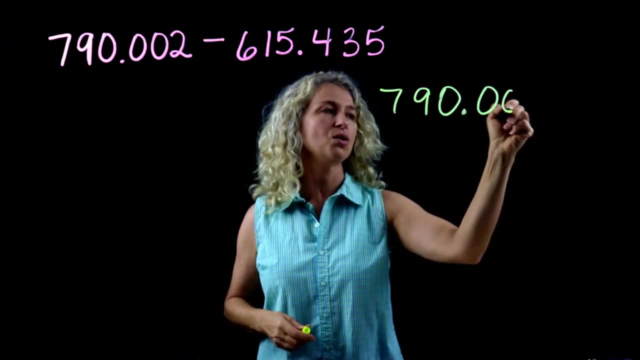 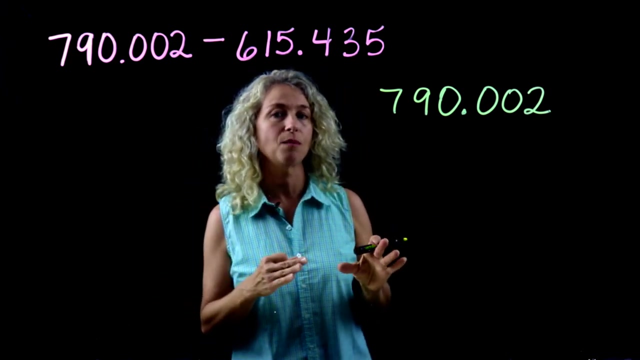 with it written horizontally. We need it to be vertical, All right, so let's rewrite the number seven hundred ninety and two thousandths And every single time when you're writing your subtraction problems, your first number is going to be your top number. okay, So write it on. 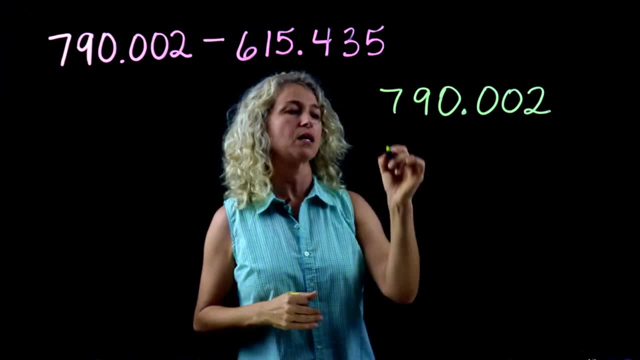 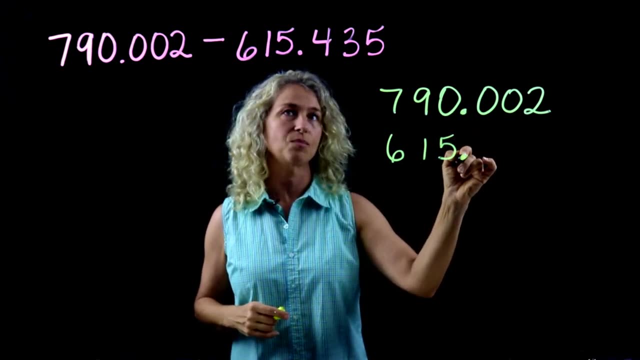 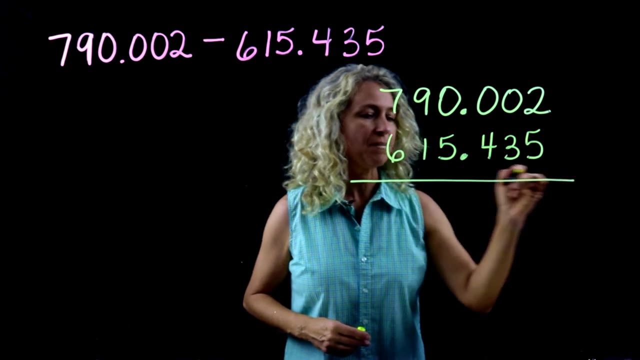 top. It's going to have the greater value when it's written horizontally. Write your number underneath: six hundred fifteen, making sure that you're lining up your decimals, and four hundred thirty-five thousandths- okay. Now that's critical. to write it correctly and make sure. 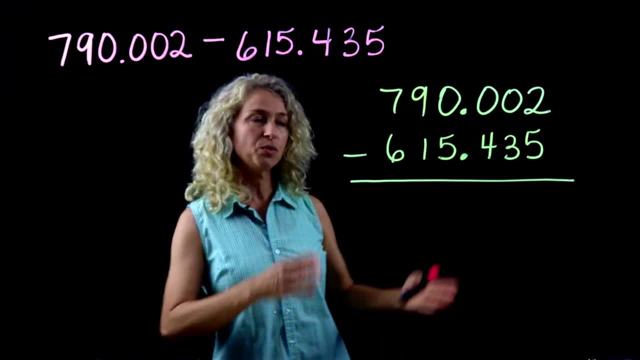 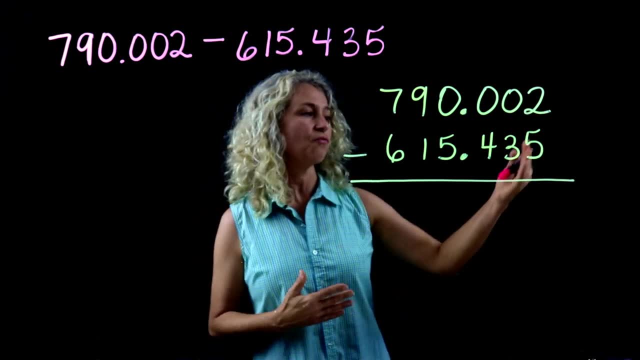 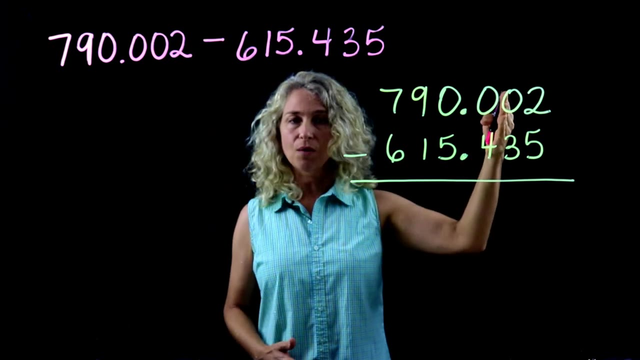 these decimals are lined up, All right. so after we have our number lined up, the decimals are lined up. now we can subtract like usual. So we're taking five away from two and we know we can't take them all away, So we're going to have to borrow. You can't borrow next door, you can't borrow next. 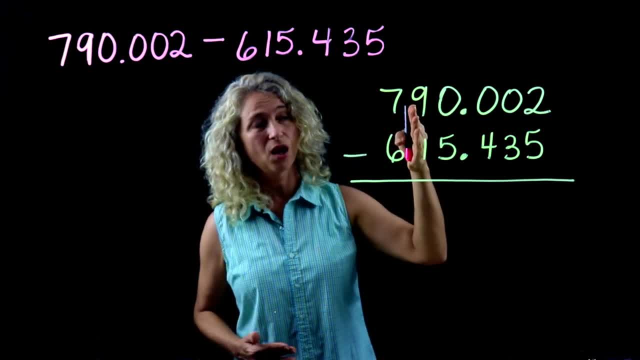 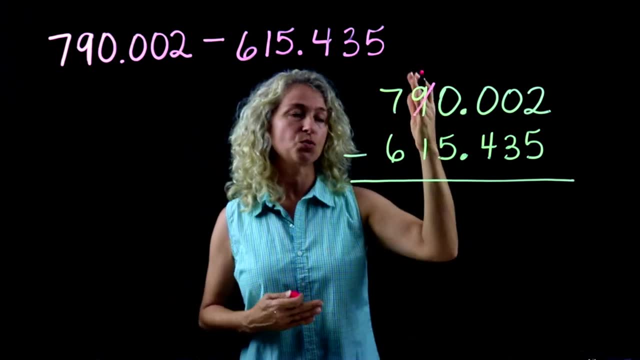 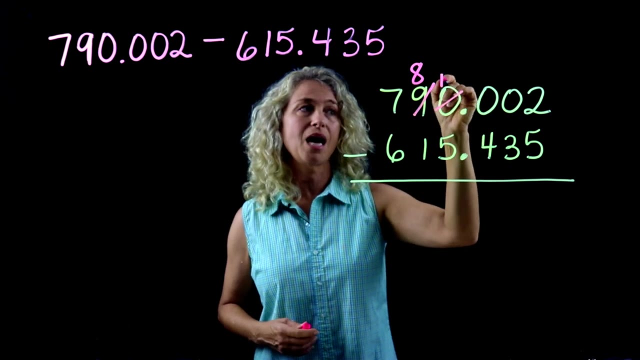 door and you can't borrow next door to that, So you've got to go all the way over to your ten's place to borrow, all right. So what is happening is we're taking one away from the nine and it becomes an eight, So this one is becoming a ten. okay, But we know that we still have to borrow. 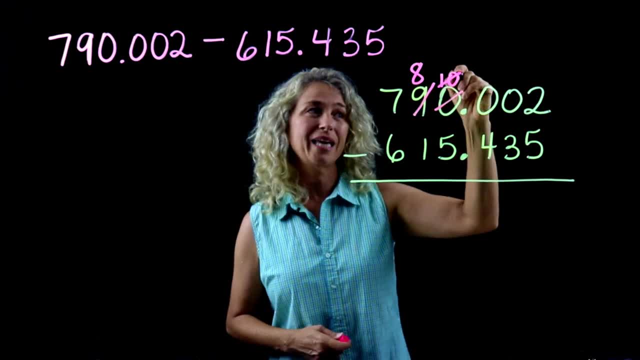 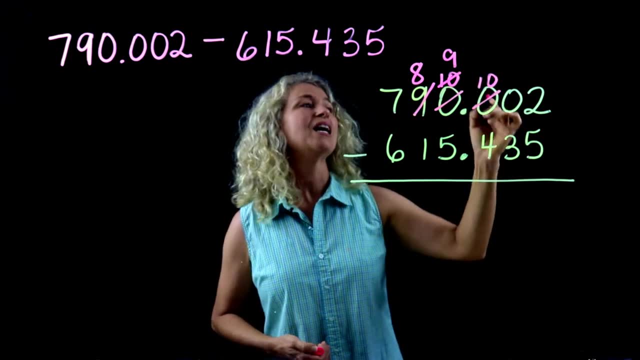 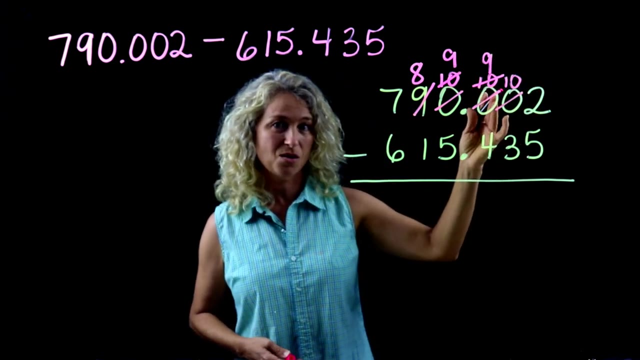 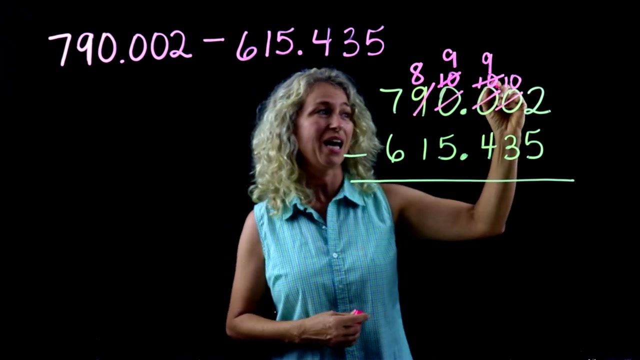 okay. So if we're borrowing, we're taking away from the ten and it becomes a nine in order to make this one a ten, right, And we're taking away from the ten and making it a nine. in order for this to become a ten, okay, And then to be able to finally get our additional ten, we have to take one away. 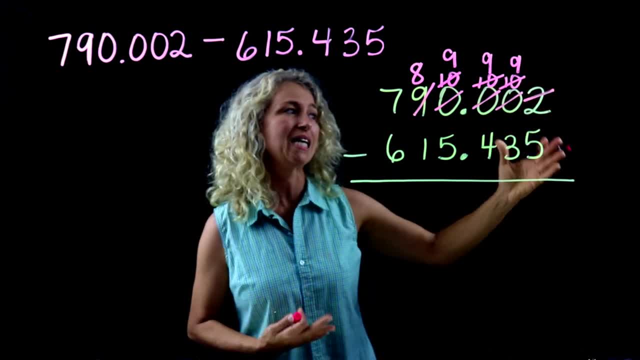 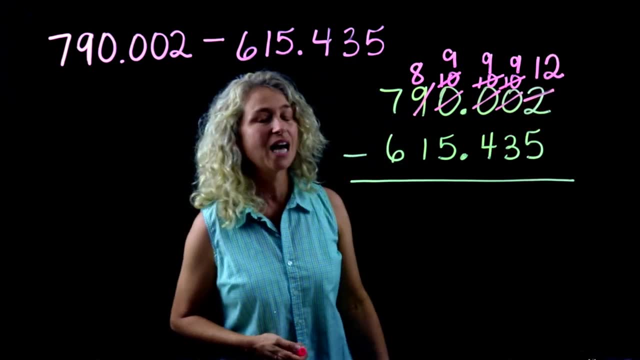 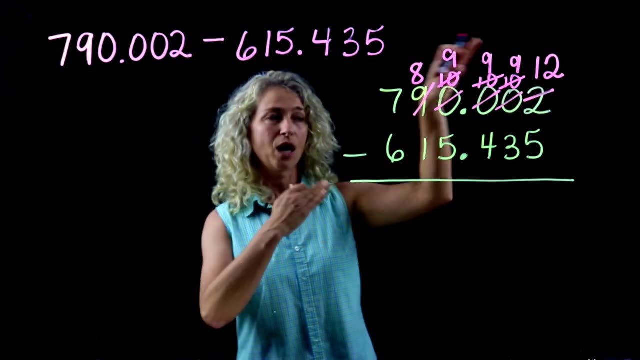 and this becomes a nine, and now we can add our ten to our ten. So, to explore these functions of how the coming of year works, what I want you to use is this new too many numbers? okay? So in order to get ready for the coming of year, 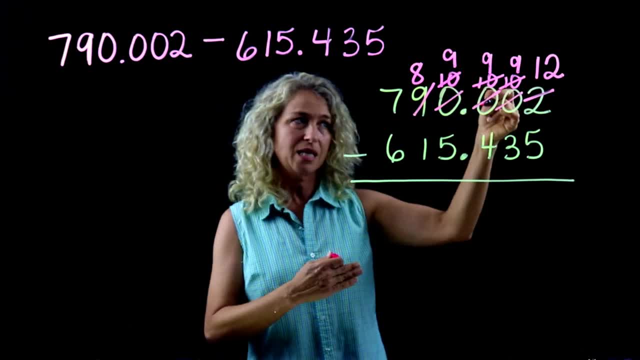 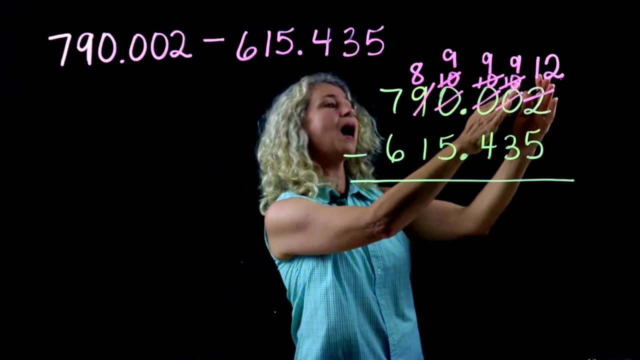 what we want you to do is we have to go over all three numbers. So what we want you to figure out is, when you go entre the rest of the numbers, you don't necessarily necessarily have to make an addition. no, we all can make additions, right, and I've written that down. 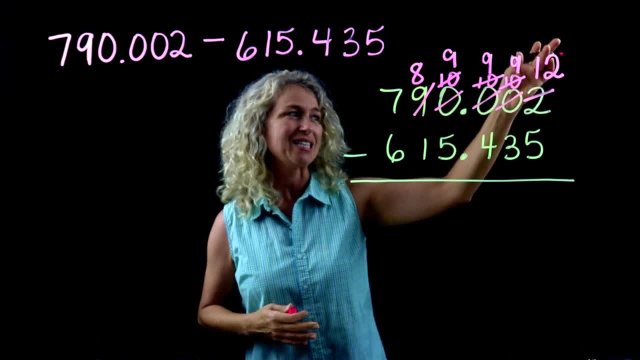 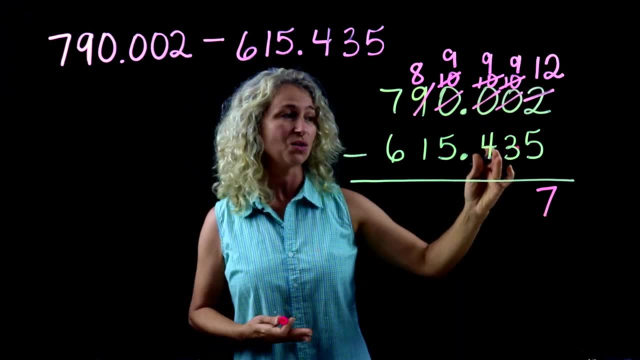 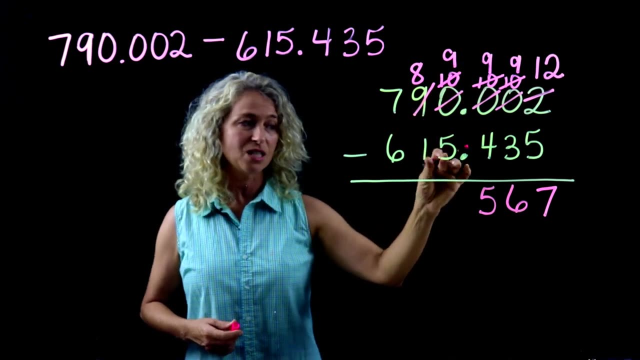 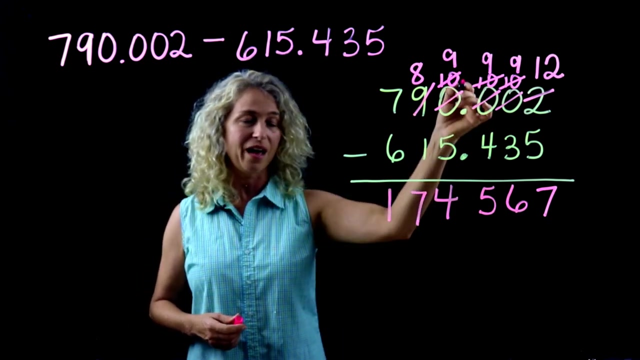 okay. so now subtract 12 minus 5, which is 7. now you can subtract 9 minus 3, which is 6, 9 minus 4, which is 5, 9 minus 5, 4 and 8 minus 1, 7, 7 minus 6 is 1, do not forget. 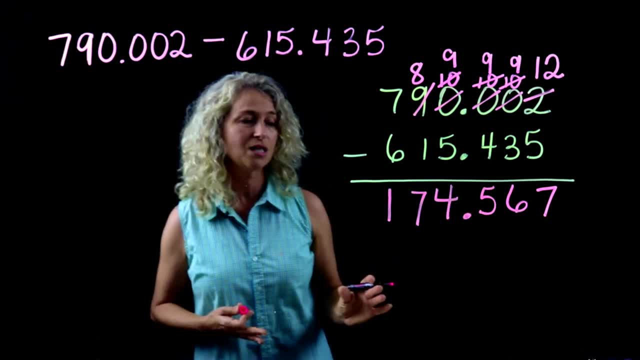 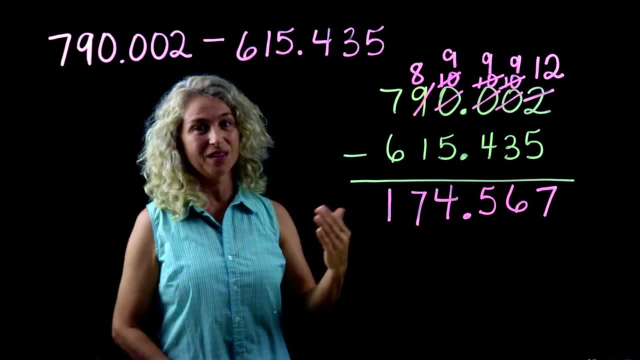 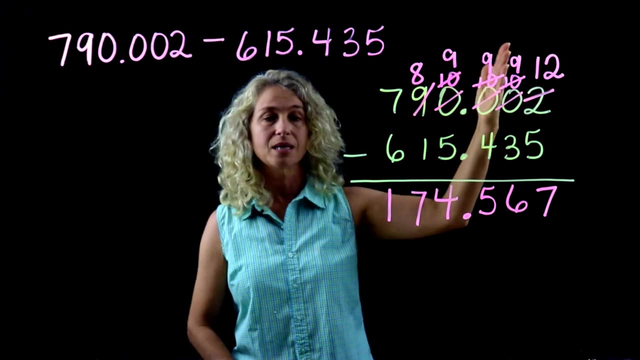 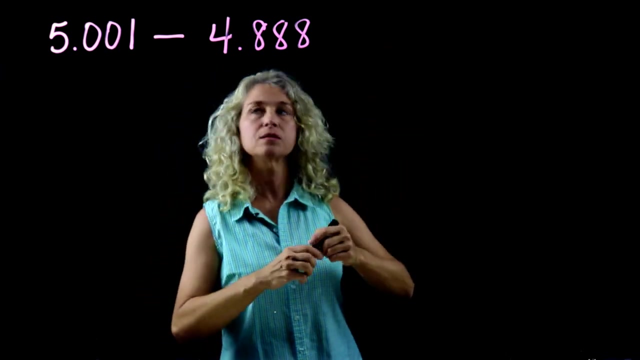 to bring that decimal down. so your final answer is 174 and five hundred sixty seven thousandths. all right, so on on this one. just to recap. notice: when you go across a zero, it becomes a nine. all right, here's our next example. let's rewrite it. let's go vertical, make sure, making sure that our decimals are lined. 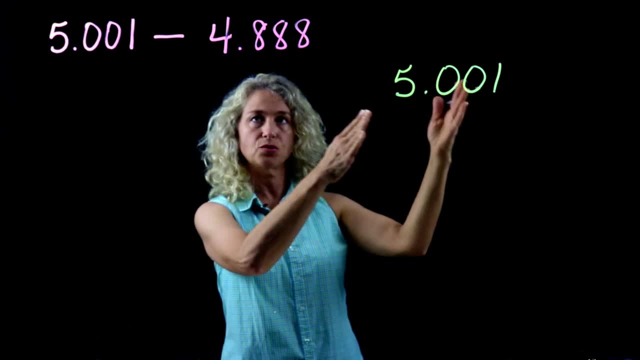 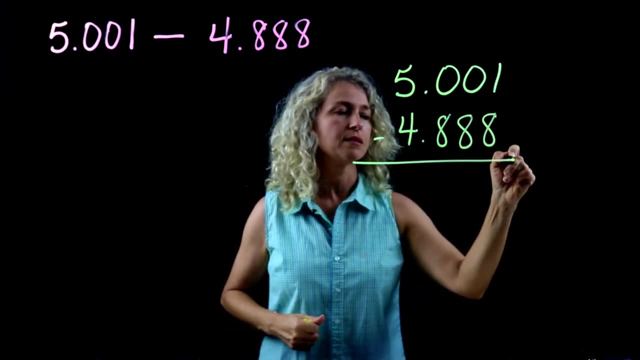 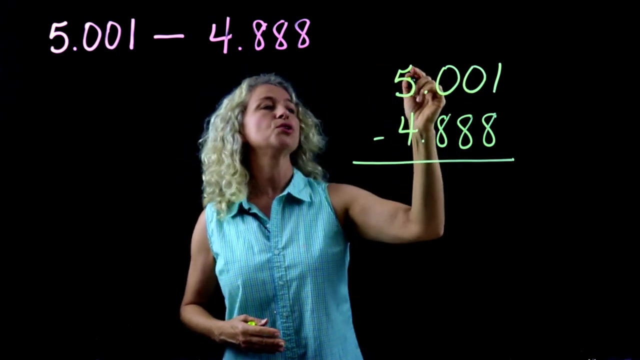 up. remember your first number is always your top number because it has the greatest value, right? so let's subtract. you cannot take 8 from 1 borrow. you can't borrow. you can't go all the way over to your ones place and make the 5. 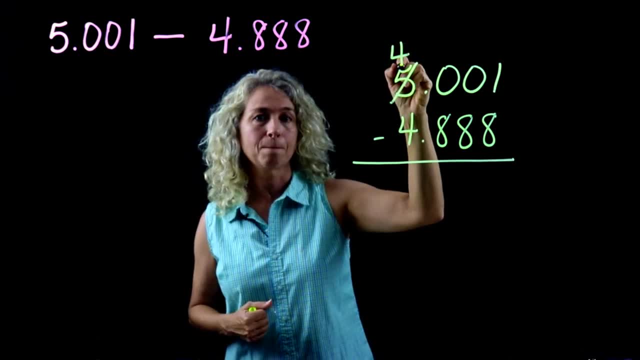 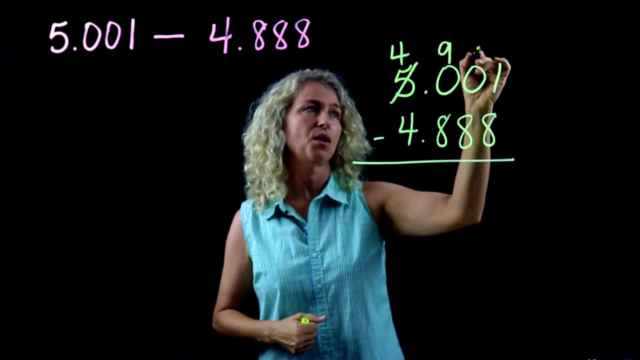 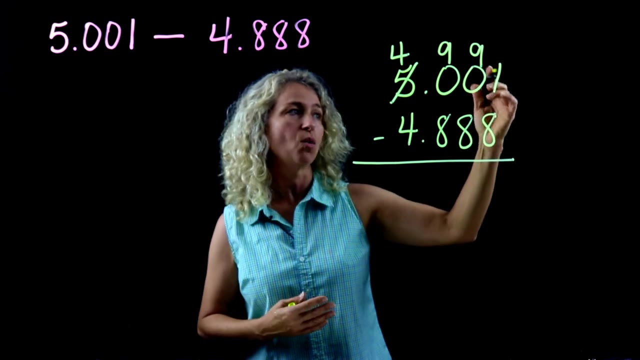 1 less, which becomes a 4. when we go across a 0, just make it a 9. we're going across a another 0, make it a 9. now here's where we're going to add the 10: 10 plus 1. 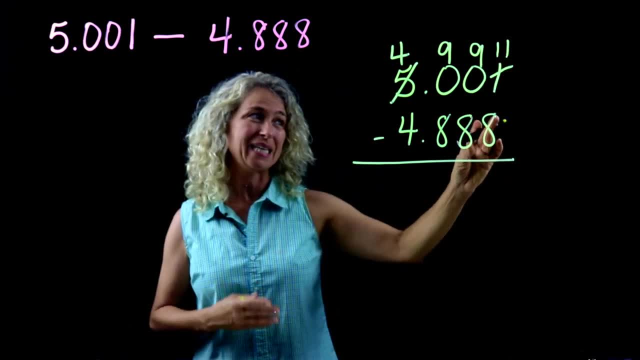 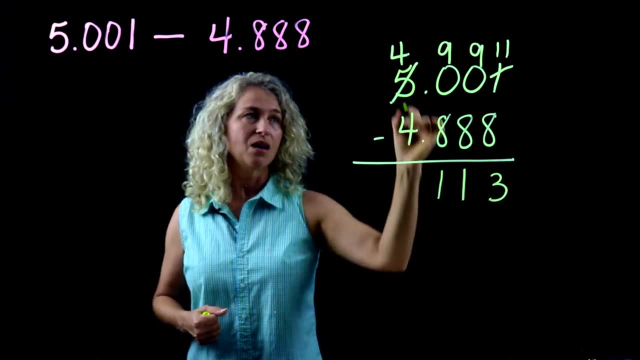 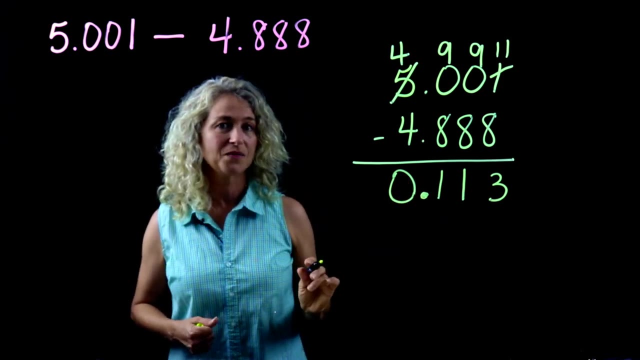 becomes an 11. 11 minus 8 is 3, 9 minus 8 is 1, 9 minus 8 is 1, 4 minus 4 is 0. make sure that you bring your decimal down, all right. so your answer is one hundred. 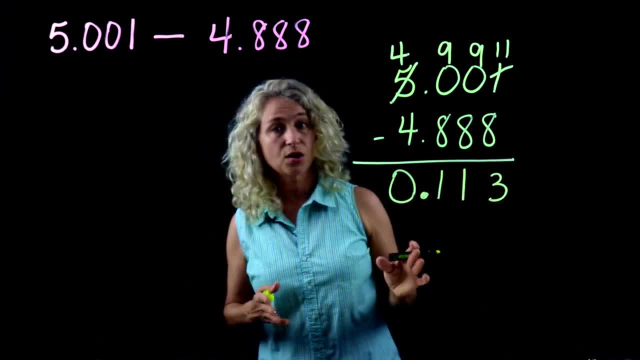 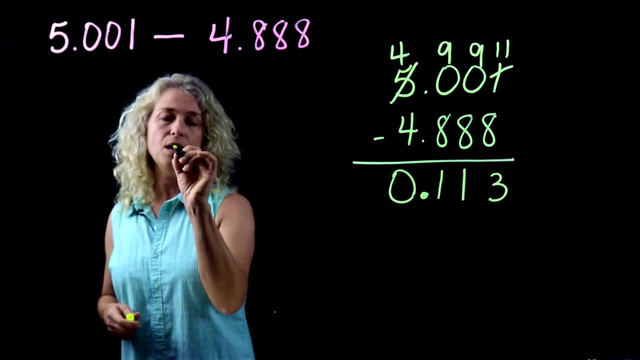 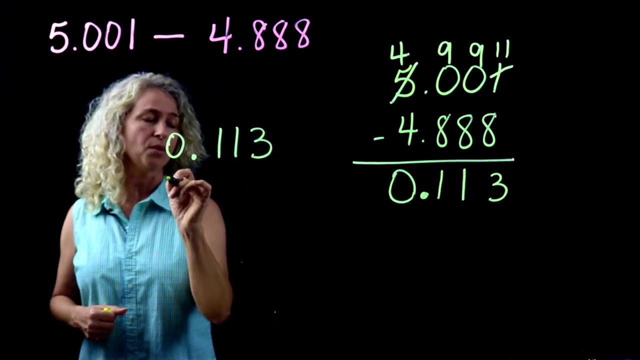 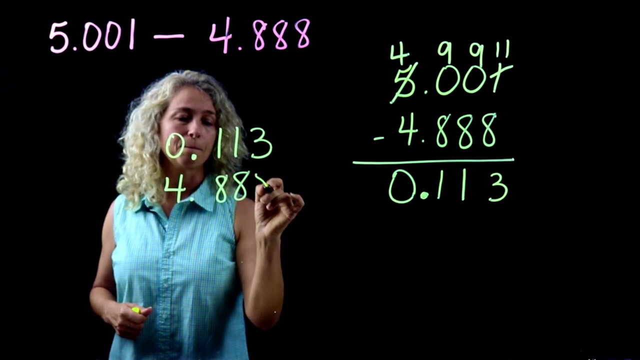 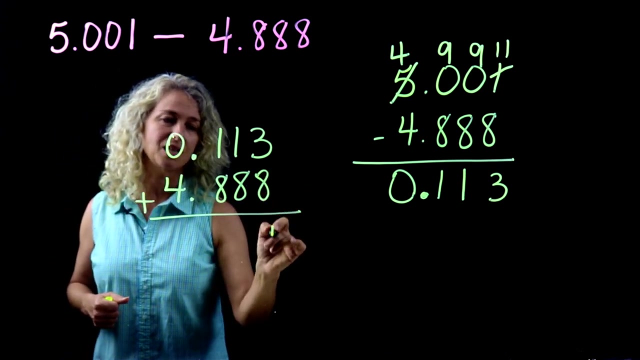 thirteen thousandths. now, could I check this to make sure that it's correct, of course, so you can take your number, your final answer, and you can add it back to the number above it and make sure that you get the number, your first original number, and if you do, you know you got it right. so let's add to check: eight, nine, ten. 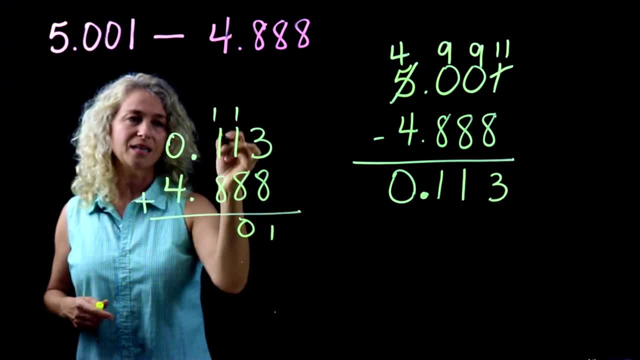 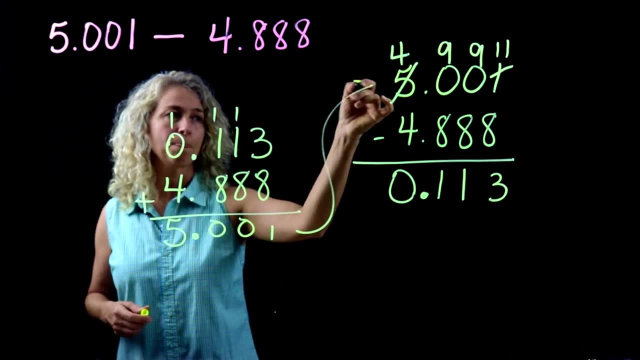 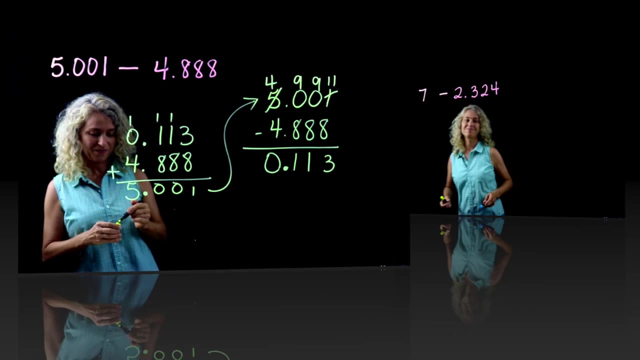 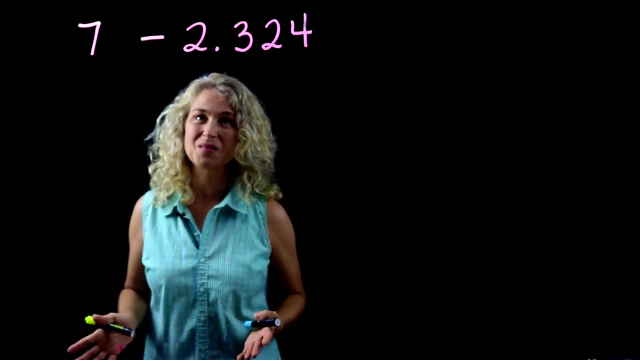 eleven, eight, nine, ten, eight, nine, ten and four plus one is five. so we got our original number and we know we got the correct answer. now. we know it's correct because we checked it. here's our last example. look at this. one looks a little different, doesn't it? you're still going to write it again vertically. 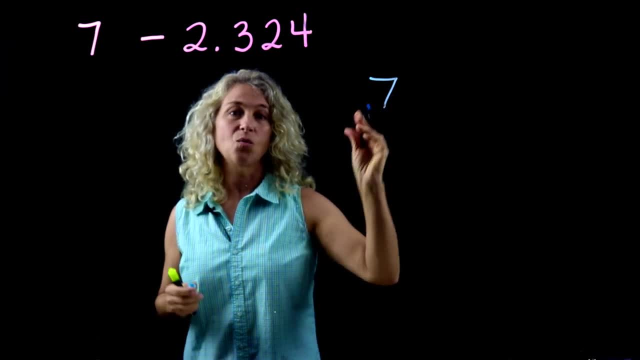 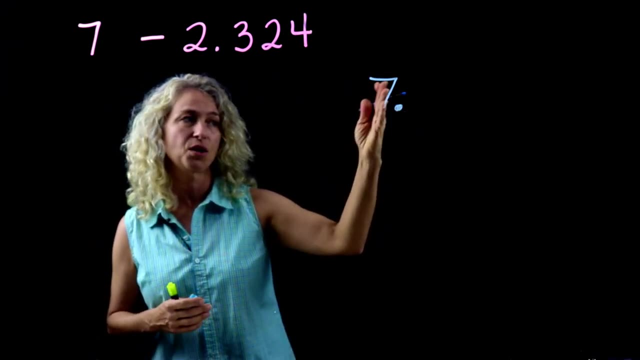 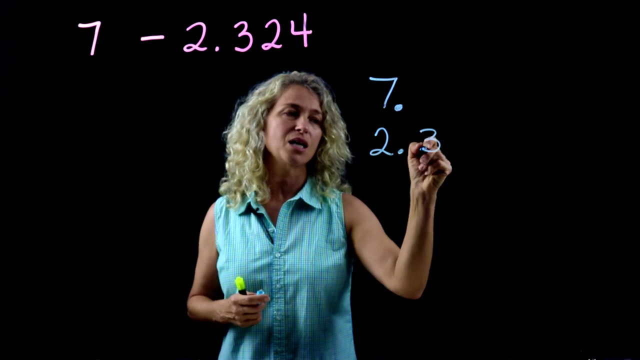 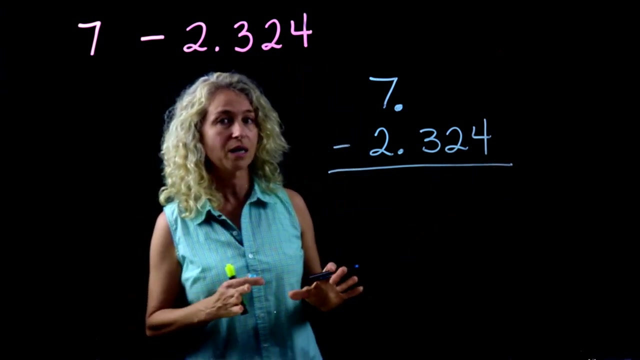 you have to know where your decimal is when it's not there, and it's always to the right of the whole number and this is your whole number one. so here's our decimal. and seven is greater than two and third, 324 thousandths. so right here, just knowing how to write the problem correctly. 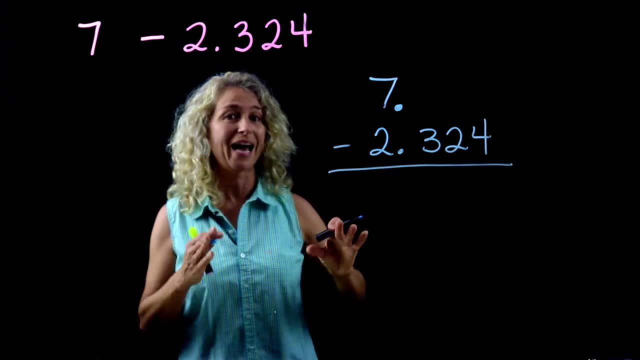 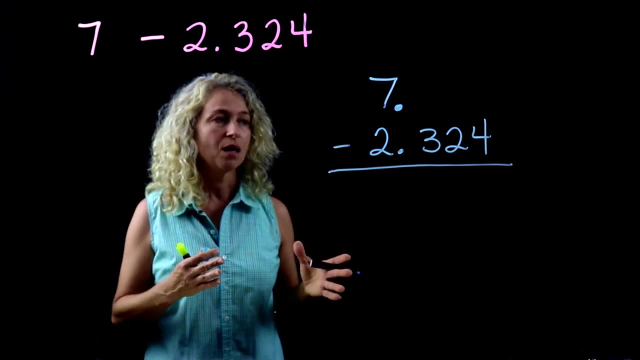 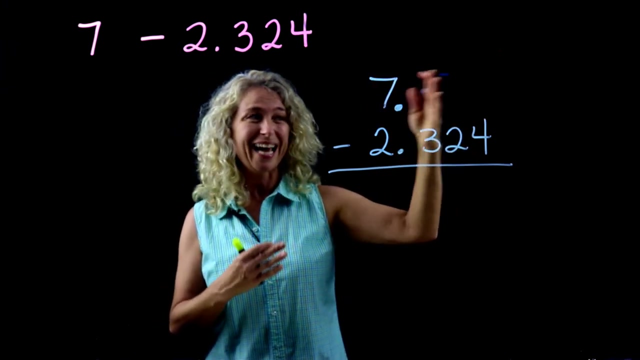 and knowing which number goes on top is half the battle. a lot of students will reverse these and then you'll end up with a negative number. all right, so seven, and if there's no and nothing above here, nothing in the tens or hundreds or thousandths place you need to fill. 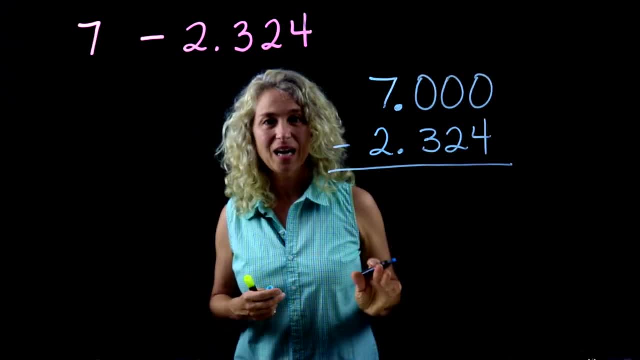 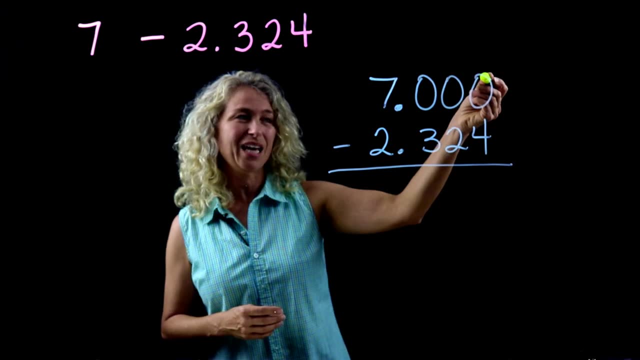 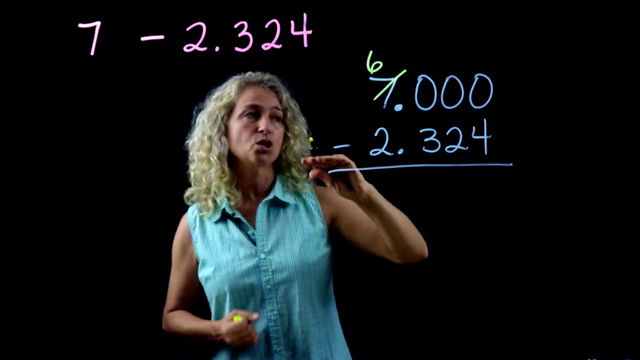 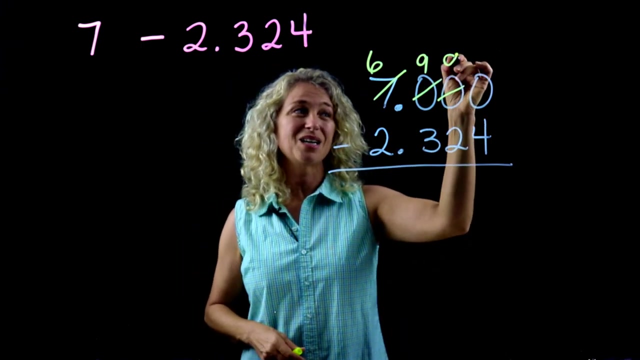 these in with zeros. okay, and now we can actually subtract. all right, so so four. can you take four away from zero? no, we're gonna borrow all the way over and the seven becomes a six. so when you go across the zero, it becomes a nine. we're going across another zero, it becomes. 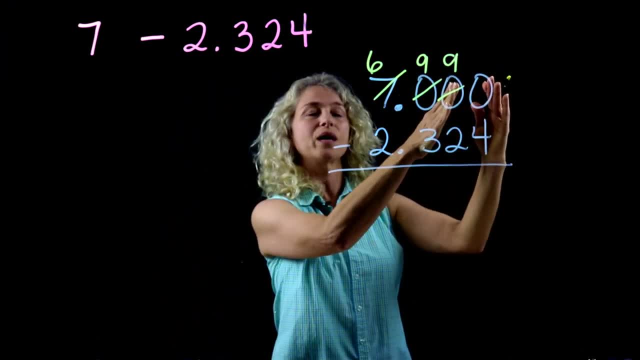 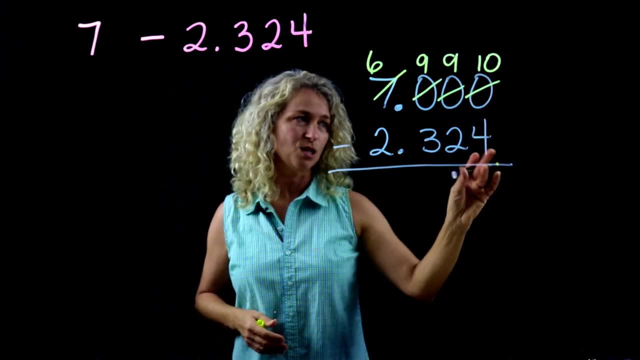 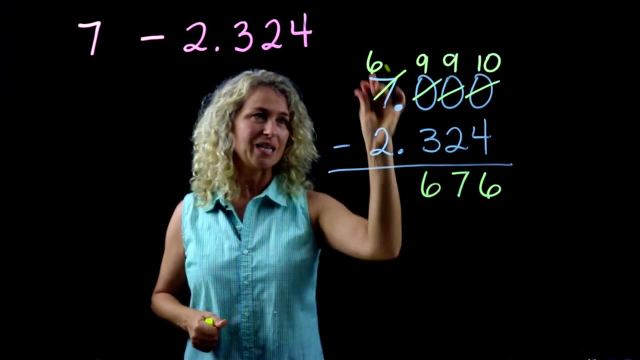 a nine, but now we're stopping at a zero and this one is going to become a ten. ten minus four, and now we can subtract: ten minus four is six. nine minus minus 2 is 7, 9 minus 3, 6 and 6 minus 2 is 4. do not forget to bring your decimal. 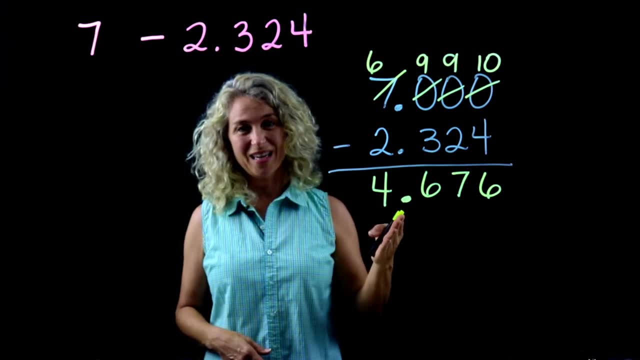 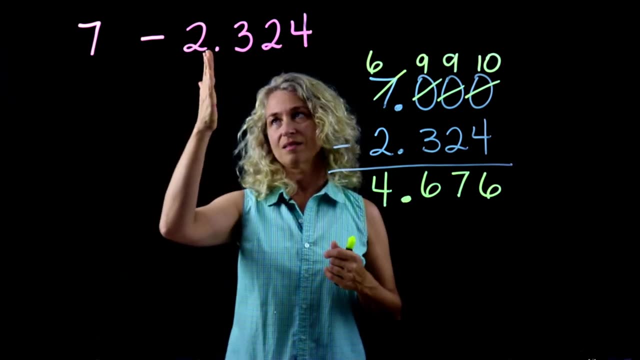 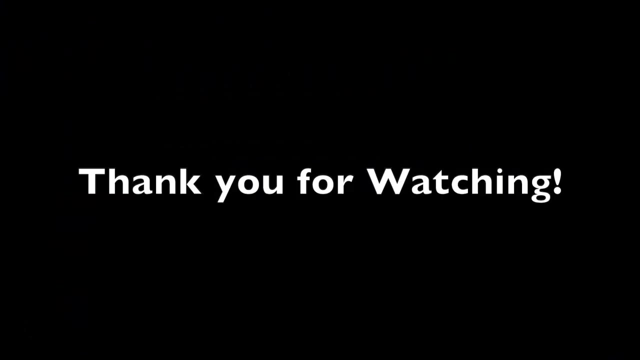 down. so 4 and 676 thousandths is your difference from 7 and 2 and 324 thousands, all right.